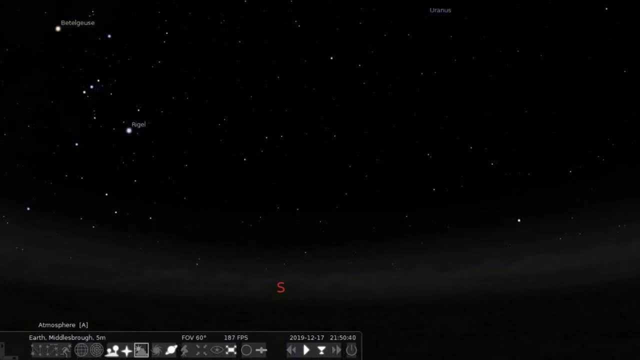 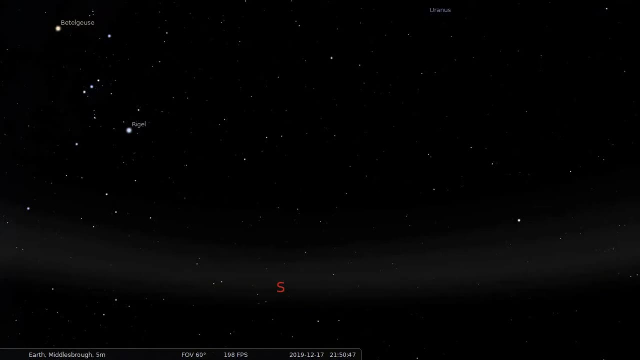 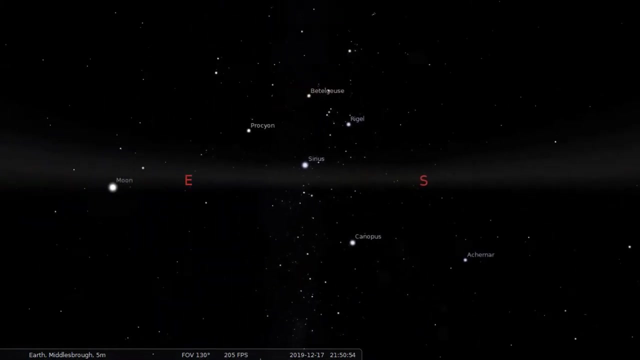 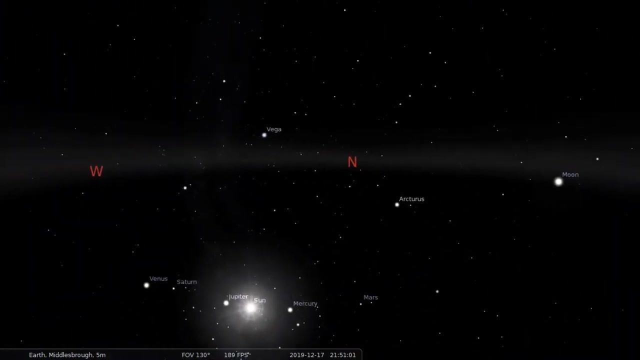 see the stars a little bit better. I'm also going to get rid of the ground so that we can see what's happening above and below the horizon If I come out a bit. and when I say above and below the horizon, because what I'm interested today in is the sun, And here we see the sun is below my horizon. 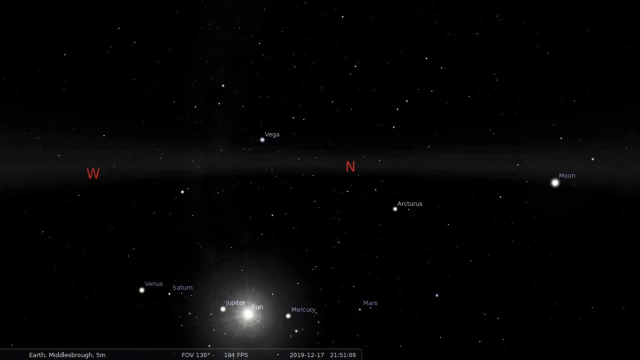 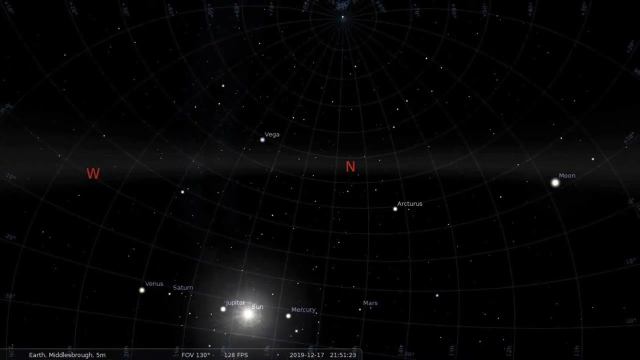 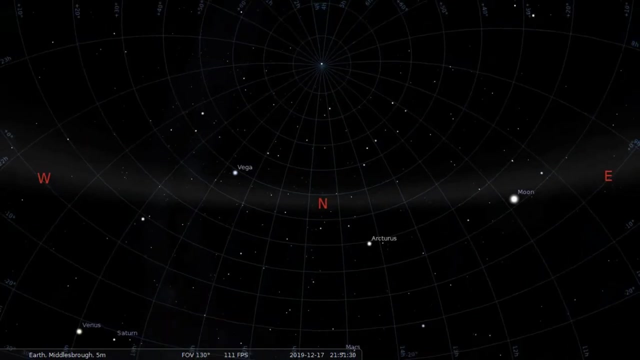 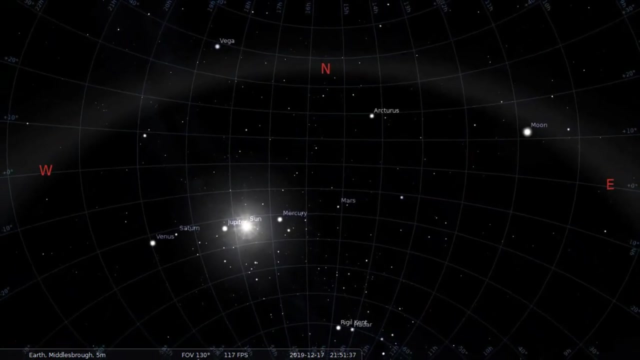 because it's night time. I'm going to add a few things to this. I'm going to add an equatorial grid So we can see right ascensions and declinations on the celestial sphere. There's the northern celestial pole up there. I'll put it so that the celestial equator is going through the middle of. 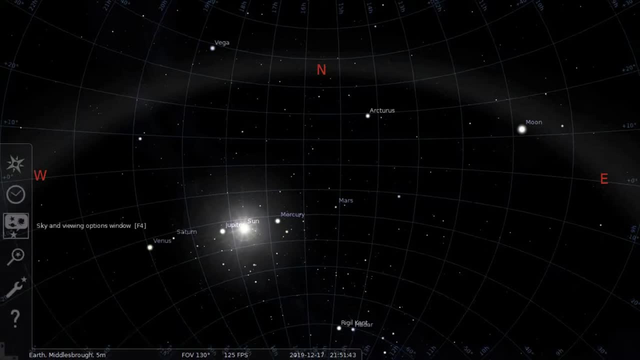 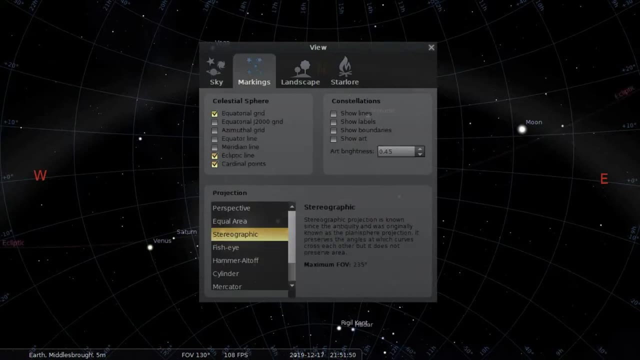 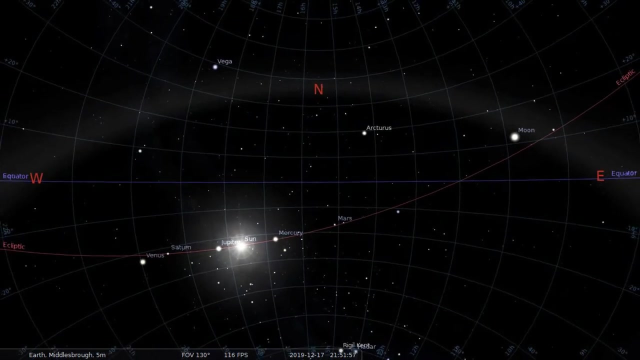 the screen, And one thing I can do with Stellarium is I can highlight the ecliptic and the equator. So this blue line through the middle is the celestial equator, which is directly above the Earth's equator. The red line is the ecliptic and that is the path of the sun throughout the year. So it's 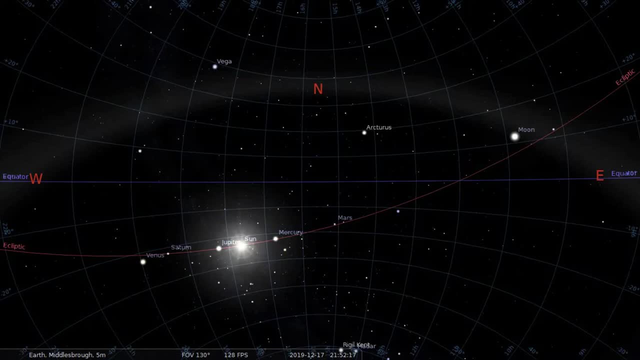 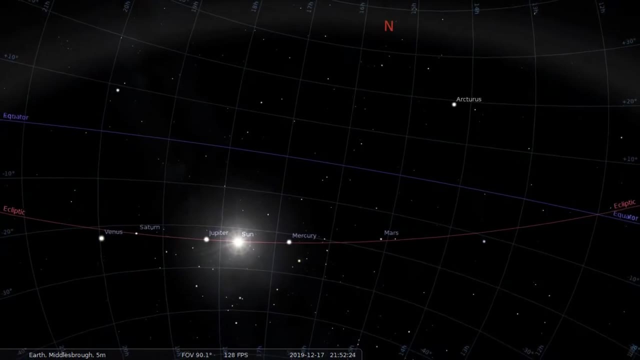 about the middle of December, The sun is well below. In fact, in about a week's time, in a week's time, the sun will be at its lowest point below the celestial equator. It will be the winter solstice in about a week's time. 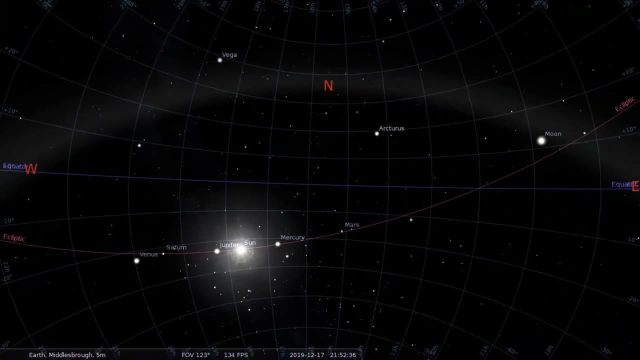 One thing you should notice straight away is that the planets are all pretty close to the ecliptic. They all happen to be kind of around where the sun is at the moment, which is interesting. Not all of them, but certainly the ecliptic. 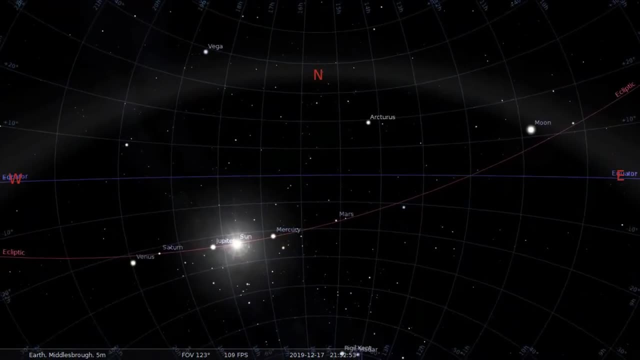 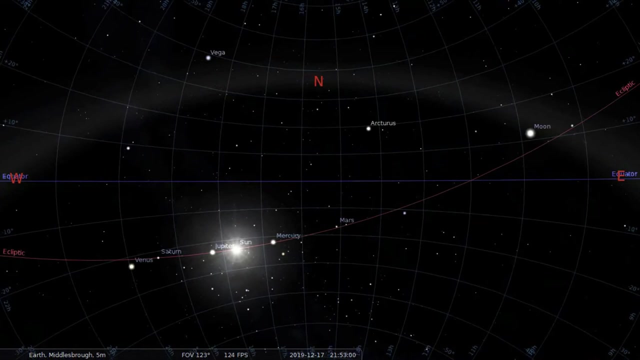 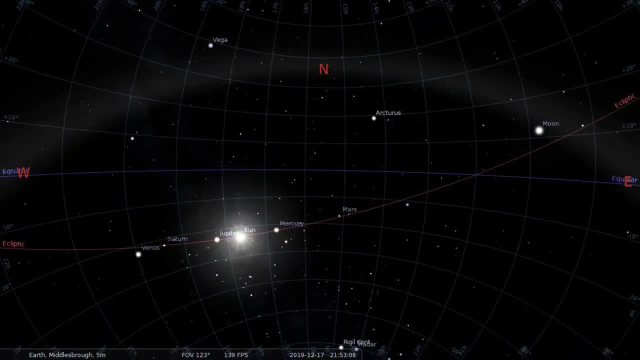 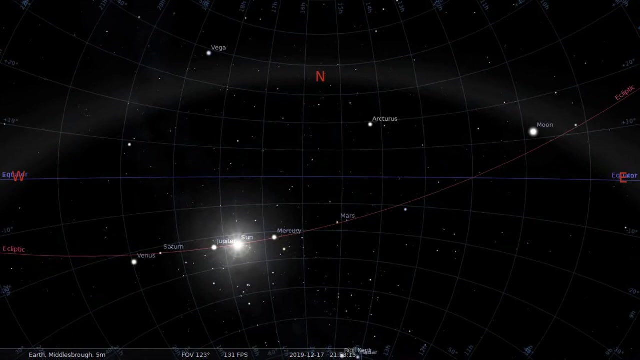 Not exactly on the ecliptic, because the orbits of the planets aren't always on the ecliptic. Some of them are a little bit inclined. See Venus. the orbit of Venus is inclined a bit. The Moon is pretty close to the ecliptic. 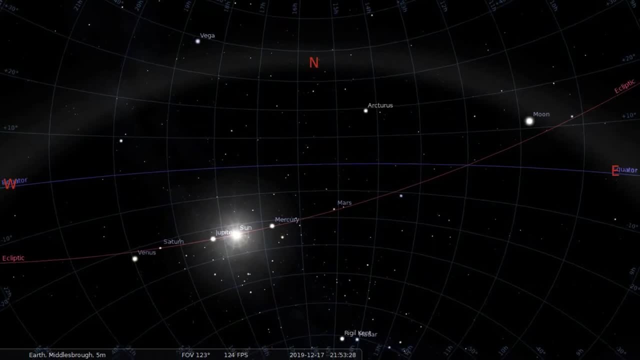 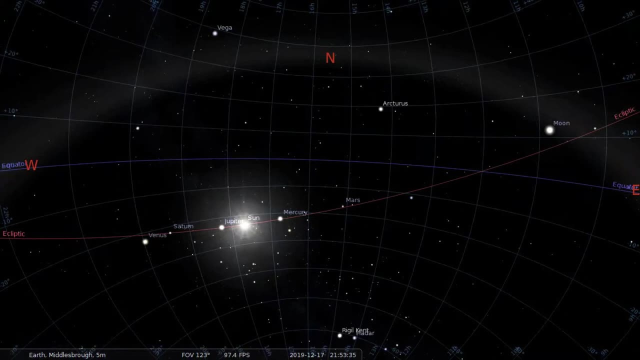 The Moon is pretty close to the ecliptic And they will take different times to go round the ecliptic. And they will take different times to go round the ecliptic, Mercury, I believe the orbit of Mercury is about 86, 87 days it will take to go round. 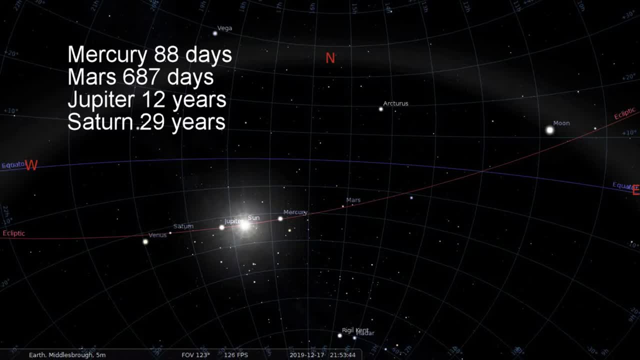 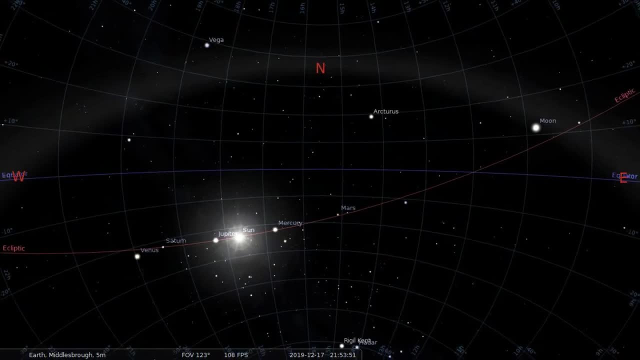 Whereas Jupiter and Saturn will take years and years to go round, Mars will take certainly more than a year. Mars will take certainly more than a year. Now what I can do is speed things up a little bit. But if I just speed it up, 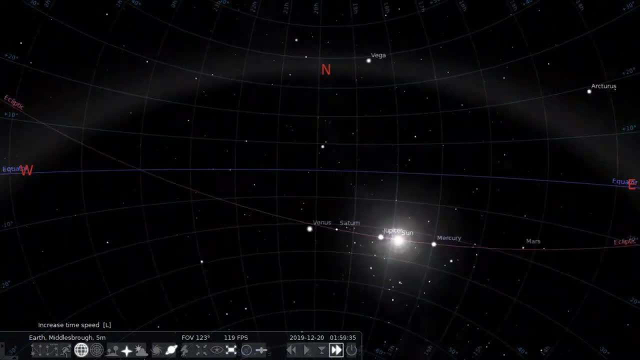 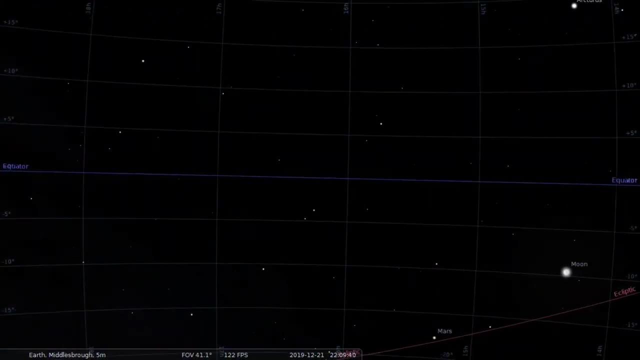 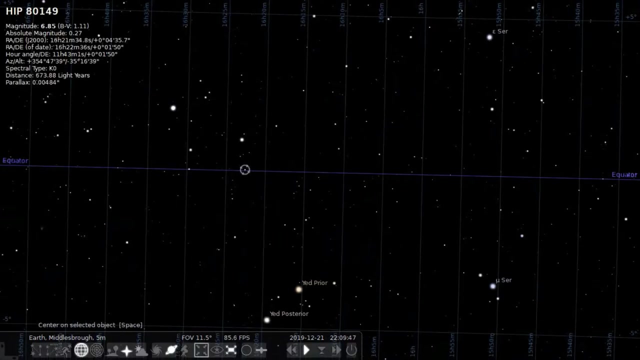 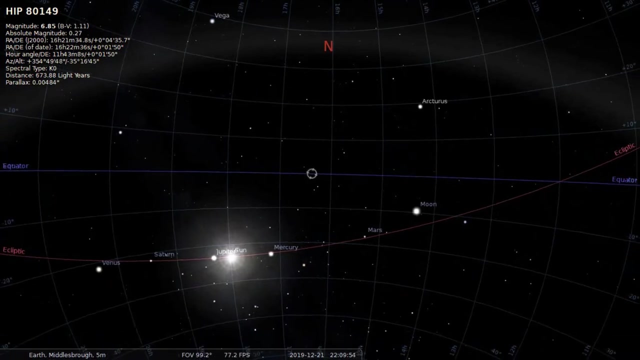 like this, then we're not going to see a great deal, so. So that's not much use. So what I'm going to do is choose a star which is pretty much on the celestial equator, and I will get it. so stays in the middle of the screen, okay, and then I will speed it up a little bit. 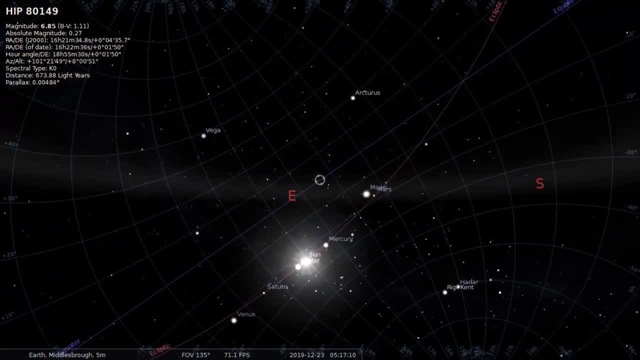 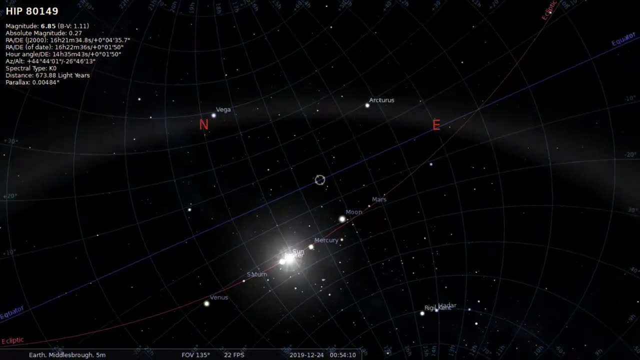 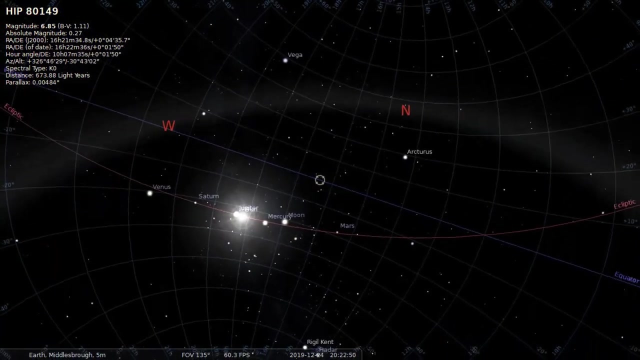 see the north, east, south west, going round as the earth rotates, the tilting due to the tilt of the earth, and, as I'm doing this, oh look, the moon's getting pretty close, so we're gonna get up. where's he gone? where's he gone, are we? 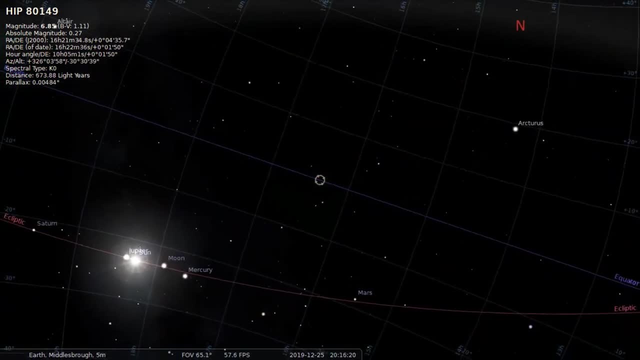 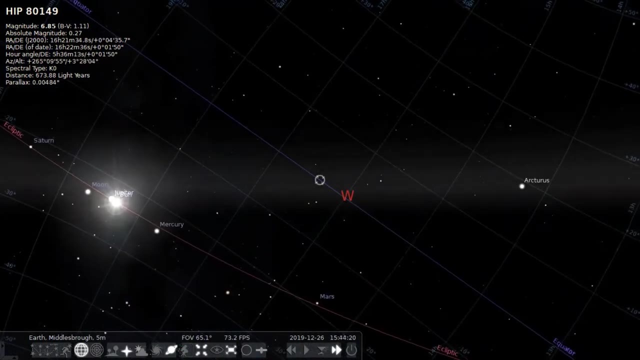 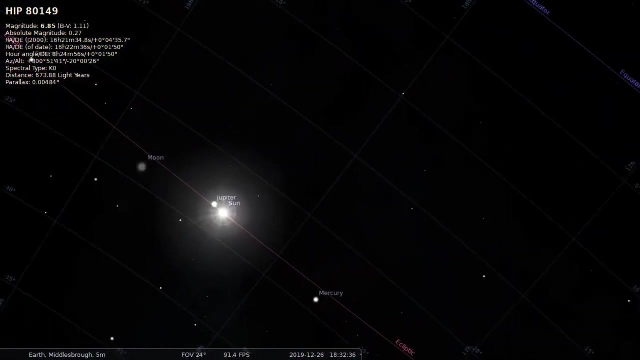 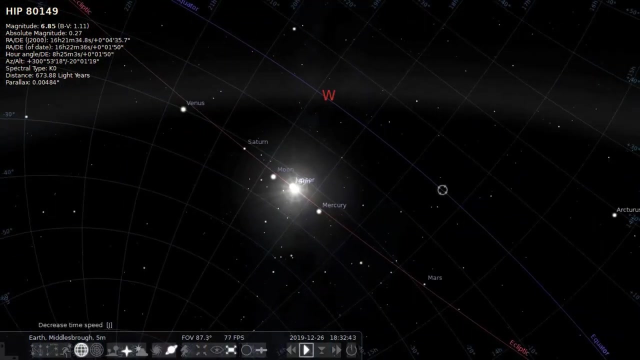 gonna get a an eclipse, no, eclipse, eclipse. no, didn't get an eclipse this time. if I stop it, you can see the moon didn't quite go in front of the Sun, never mind. no total eclipse this year dawn. we'll have to wait another hundred years or so for that. let's get back. 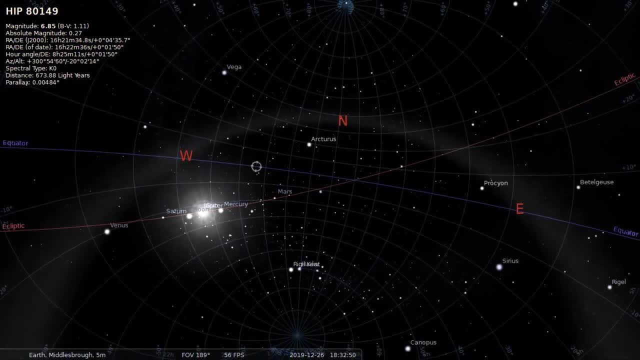 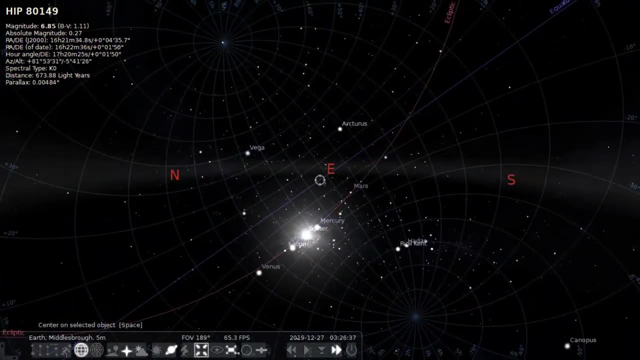 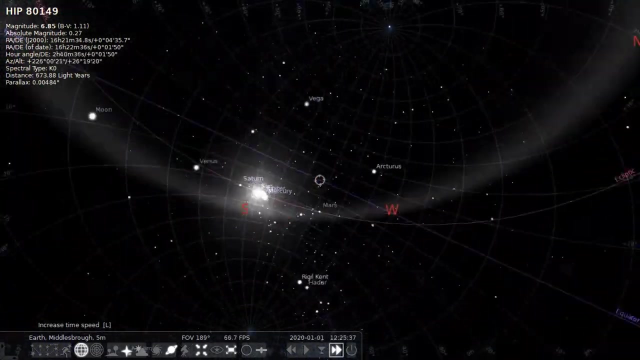 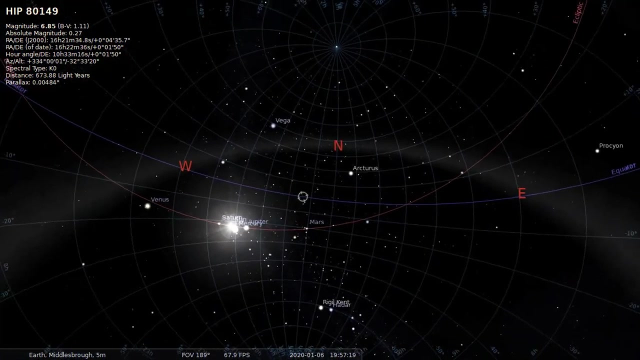 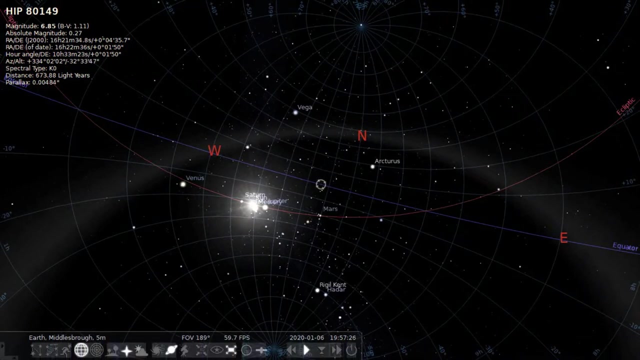 again. let's get my, get my tilting going again. Center on that star might get a bit dizzy now as the days pass. moon's long gone. stop it now. see where we are. the Sun is on its way back up up the ecliptic, heading towards the celestial equator. speed it up again. 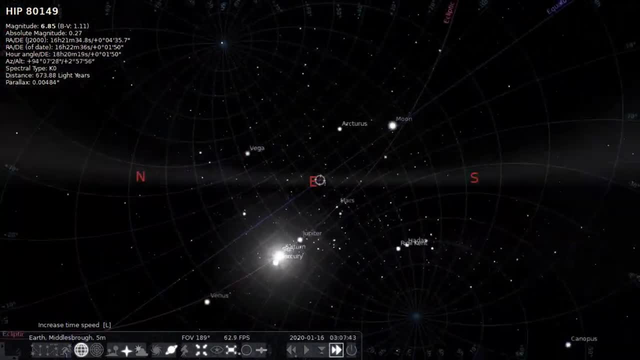 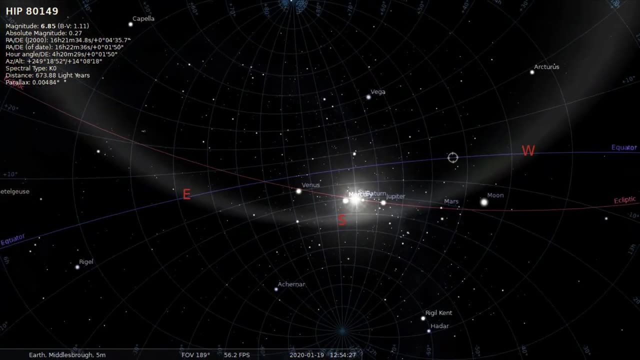 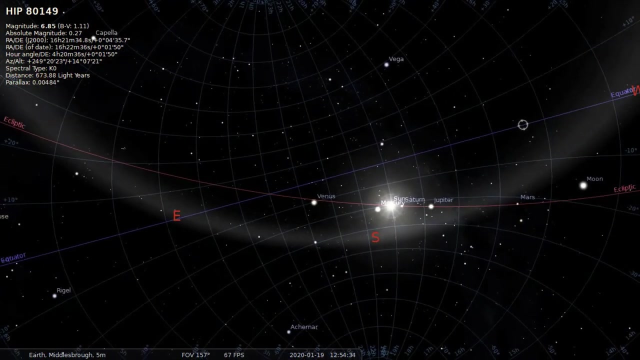 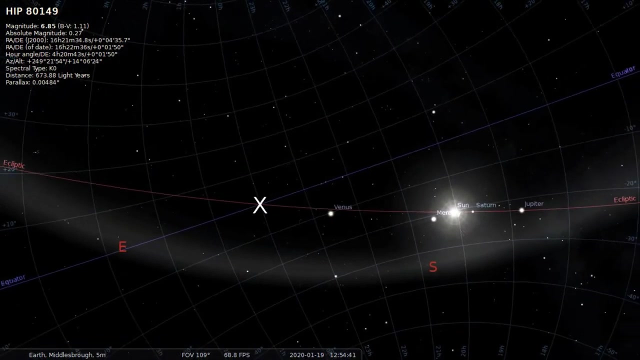 give it another couple of weeks. the vedatusha 2021. do the sun's well on its way, Venus is obviously making very good progress. this point here is very important. this, this point here, is called the first point of Aries, and it's where the ecliptic crosses the celestial equator. when that 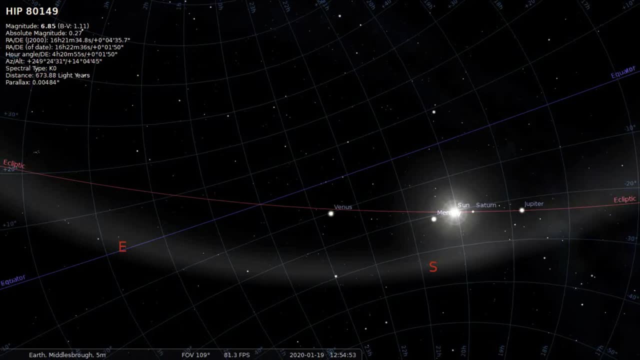 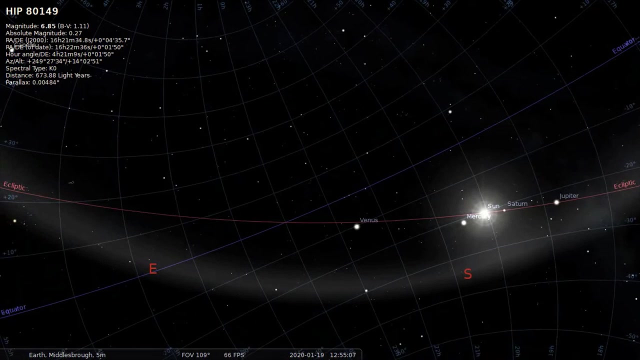 happens this: it'll be about March the 21st, and that will happen on the 화 moistly- northwest всё that will be the spring equinox or the vernal equinox, um, when hours of daylight and night time are equal. the vernal equinox, it's also the, the zero hours, zero hours of right ascension, it's a. 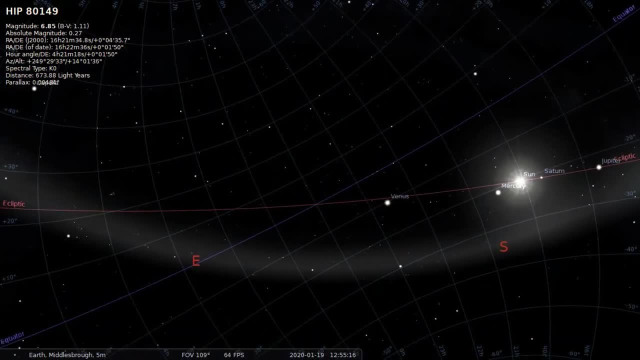 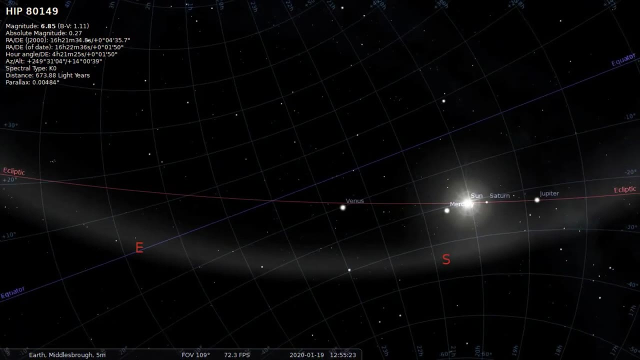 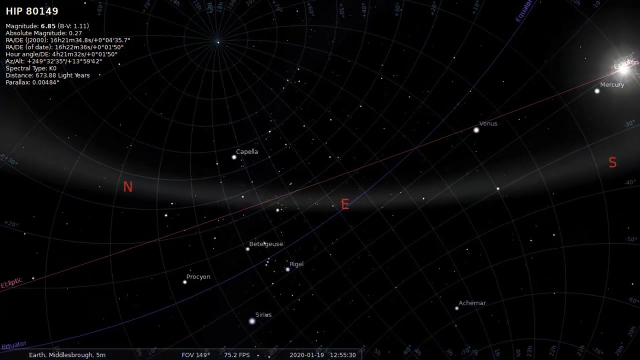 little bit like our greenwich in the sky, if you like, as longitude zero longitude goes through greenwich zero of right ascension goes through the first point of aries. we have a look around the ecliptic. let's have a look around the ecliptic in the middle of. 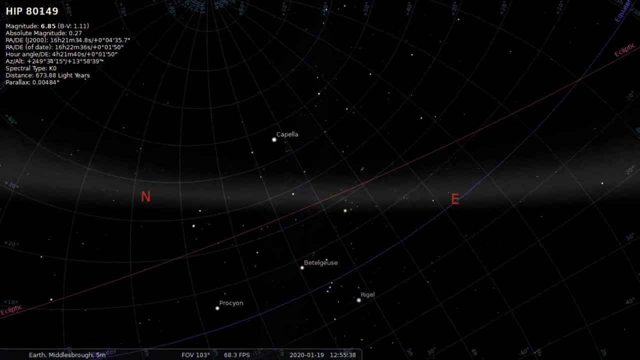 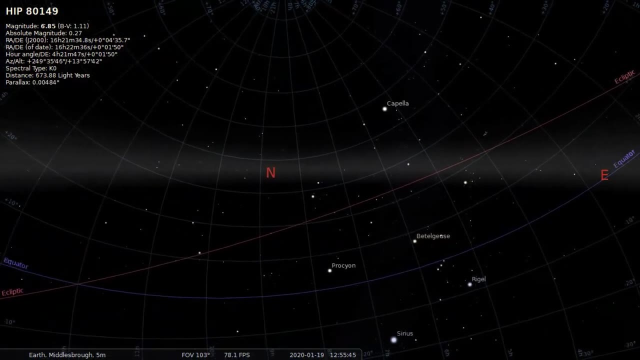 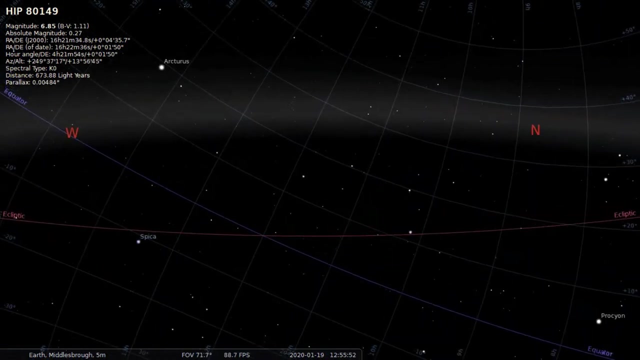 the summer. the sun will be at its highest above the ecliptic at the summer solstice. moving round at this point here, the ecliptic goes through the celestial equator on it, with the sun on its way down. that's called the first point of libra.